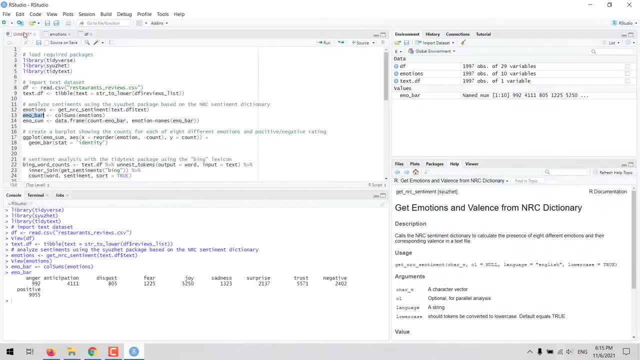 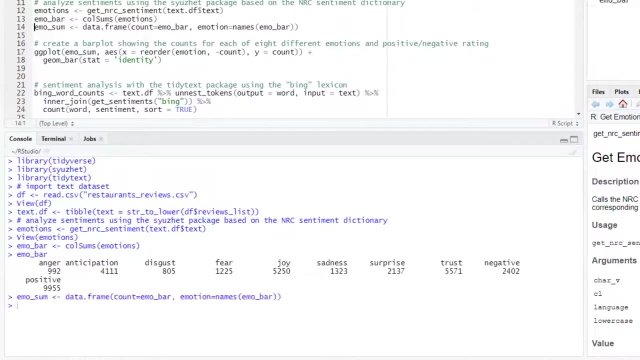 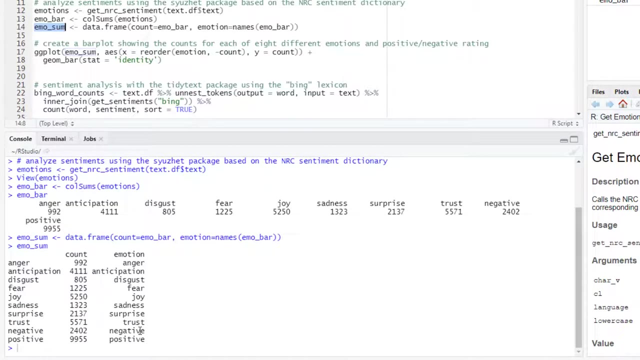 We can calculate the sum by column and then we get for each of the emotions and sentiments the total counts, and then we can make that a data frame, such that we have the counts in one column and the corresponding emotion in the second column. With this data we can create a 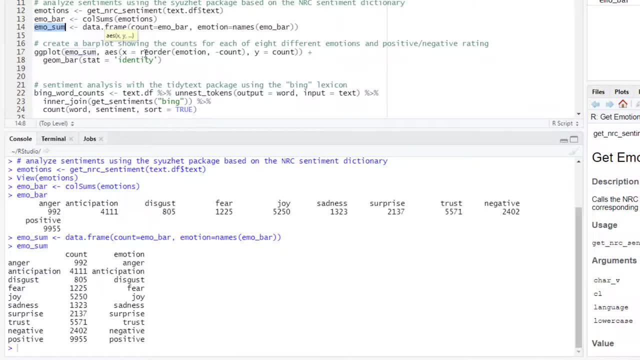 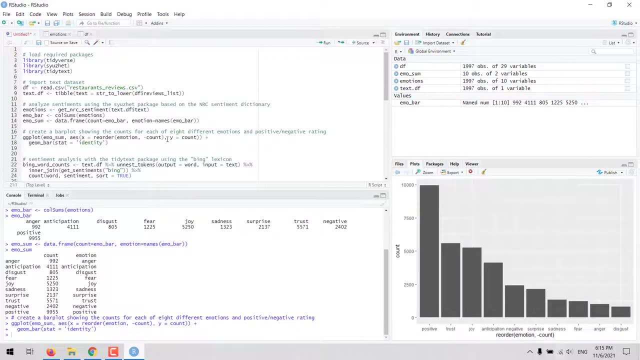 visualization. for example, we can make a bar plot with the emotion in the x-axis and the count in the y-axis. Note here that I am reordering the emotions based on the frequency, so the emotions are sorted in descending order based on the count value. In this text, data set most of the words. 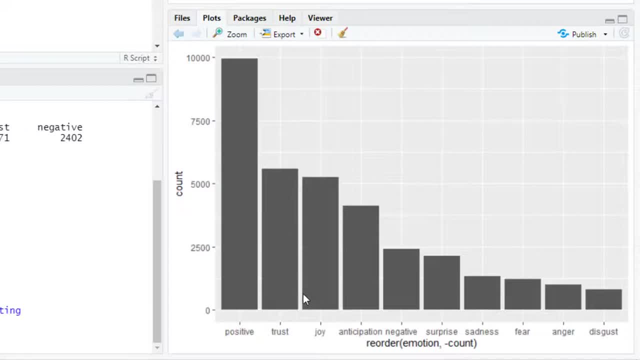 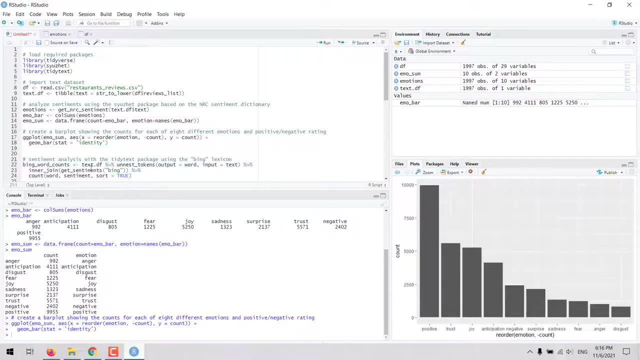 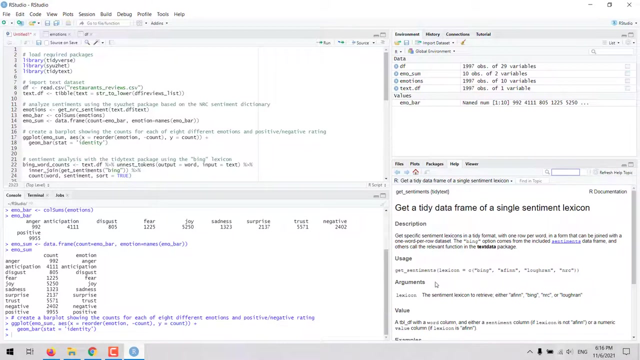 represent a positive sentiment and emotions such as trust, joy and anticipation. Now let's see an example with the Thai-DText Package. In this Thai-DText Package, the main function is get underscore sentiments. This function provides access to several lexicons, including Bing. 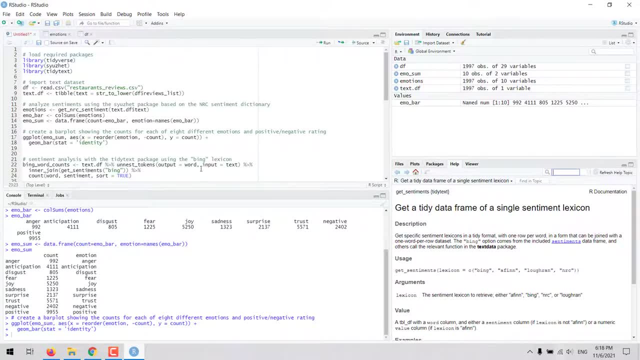 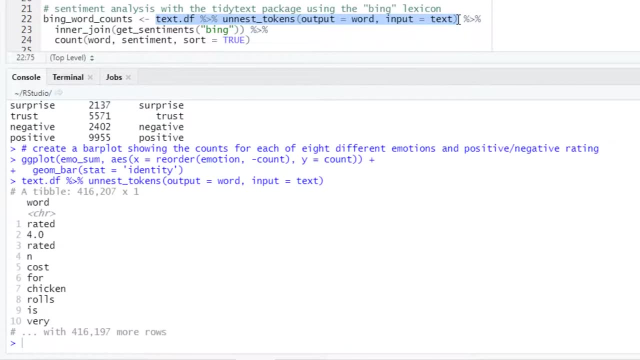 afint, LoveRand and nrc To run the sentiment analysis with this Bing lexicon. first we apply this function and nest tokens. This function creates a one-word per row data set, as you can see in the console. Once the dataset is in'stressed, all of itsomat exercises, the themes and 사랑 hai. 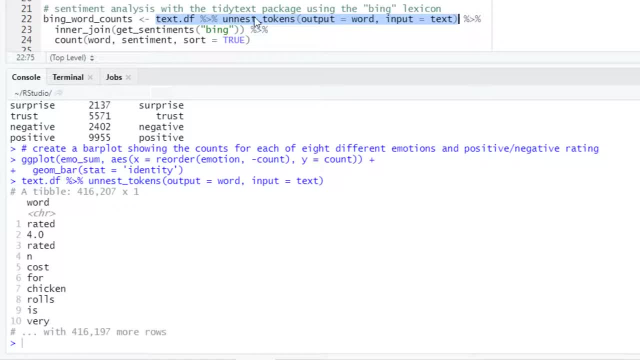 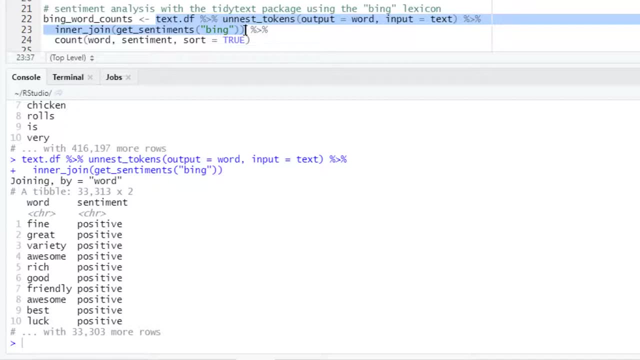 is in this tidy format. we can join it with the sentiments in the Bing lexicon and we are going to see, for each of the words in our text data set, the corresponding sentiment as classified by the Bing lexicon. Finally, we can calculate the total count, so we get the frequency for each of these words and 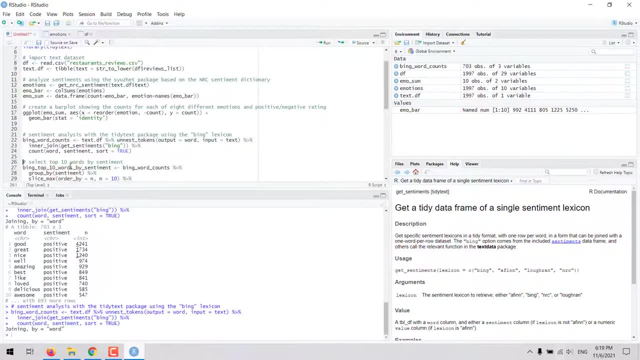 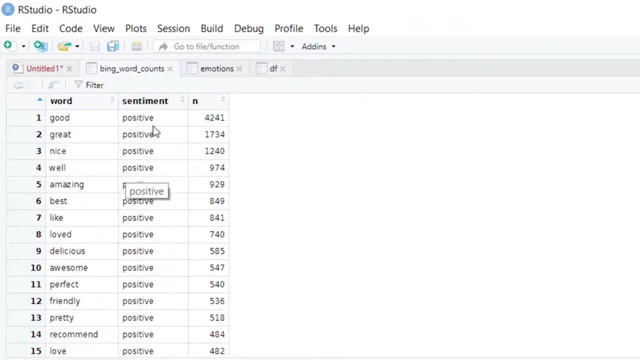 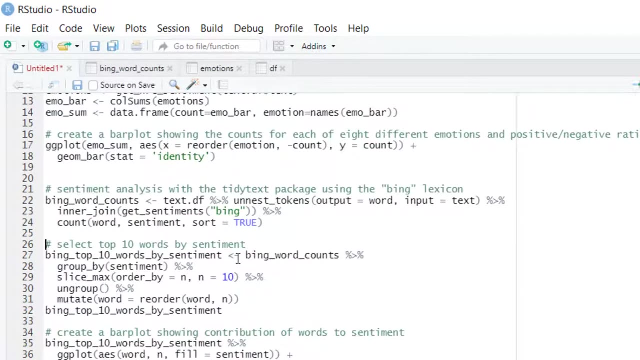 the corresponding sentiment. So let's save that as a data frame and we are going to see that there are 700 words and for each of these words we have the corresponding sentiment and the frequency. With this data we could create a visualization, but it would be better if we just select a smaller number of. 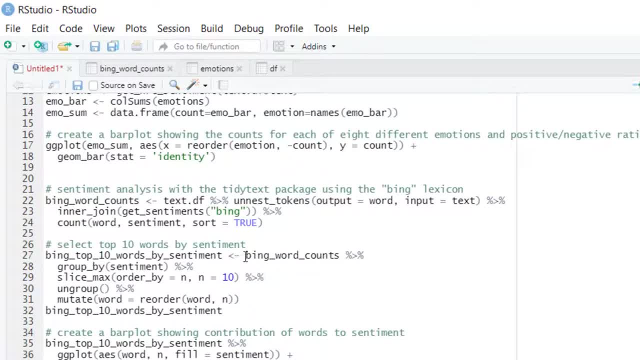 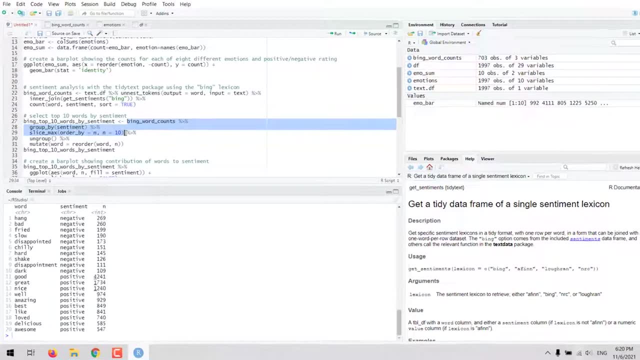 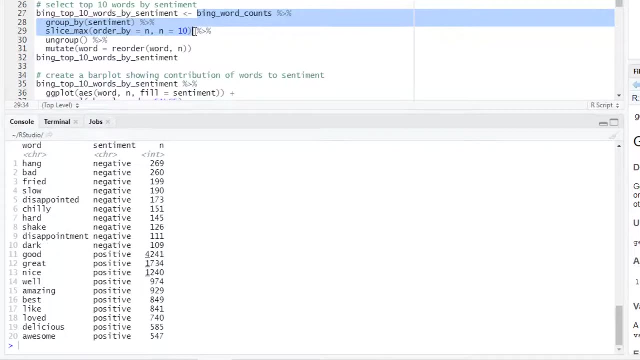 words, let's say the top 10 words by sentiment. So we can take our data frame grouped by sentiment and then use the slice underscore max function to get only the top 10 words by sentiment, that is, the words in each sentiment that have the 10 highest values corresponding to their frequency For the 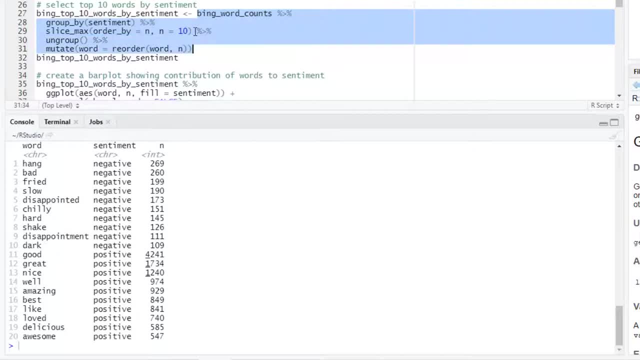 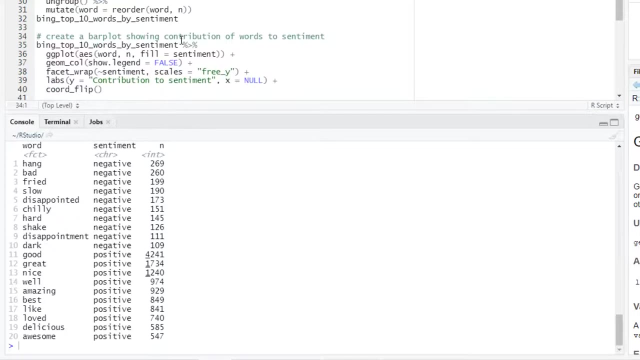 visualization. we can convert their words to factors and reorder them based on the frequency. We can use the mutate function for doing that. So let's create the top 10 words by sentiment data set and then we can create the visualization. So we can create, for example, a bar plot using the geo underscore code function and 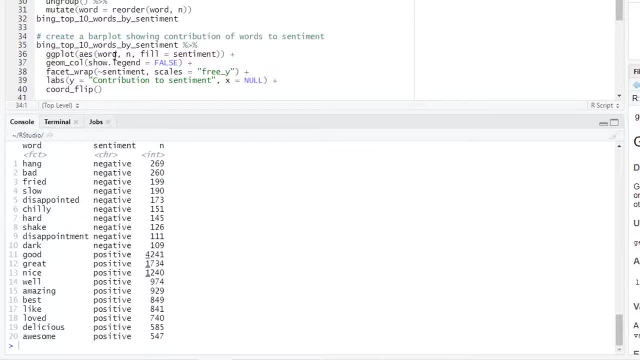 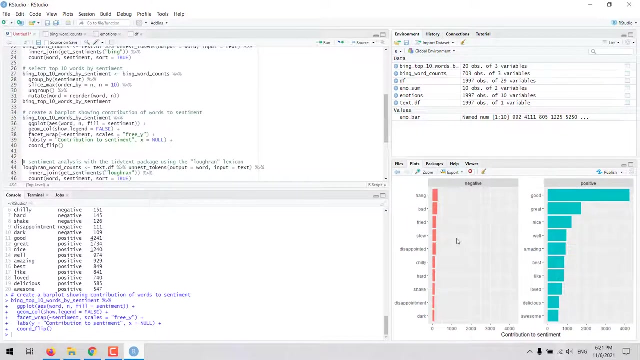 we will plot the words in the x-axis, the frequency in the y-axis, and then we can use the sentiment column for the color. If we want, we can separate that plot in two facets, as you are going to see here. So we have one facet with the 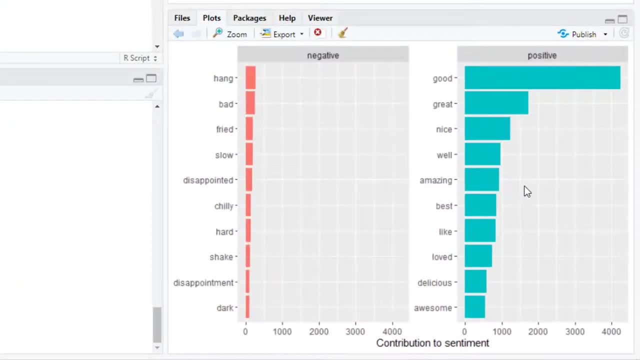 negative sentiment and another facet with the positive sentiment. We see the top 10 words that contribute to each of the sentiments. For example, for the positive sentiment, the most important words are good, great and nice, which have the highest frequency, as we can see in this. 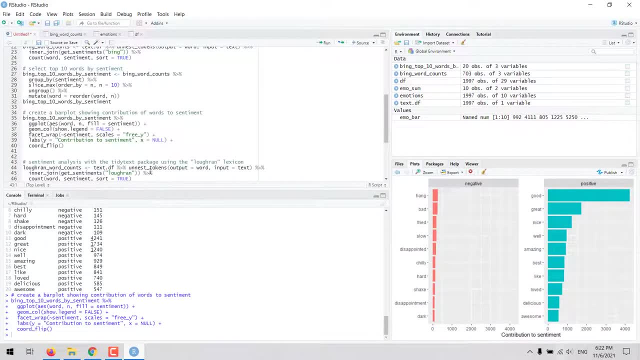 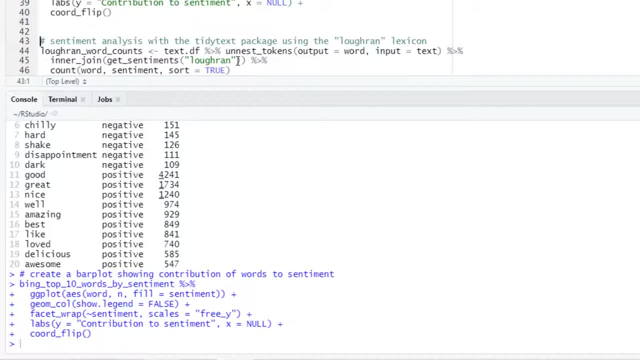 axis. In a similar way, we could do the analysis with other lexicons in the tidy text package, For example, we can use a low brand lexicon. This lexicon labels words based on sentiments that are important in a financial context. So we will do the same steps as before. We will apply the unnest tokens function, then we 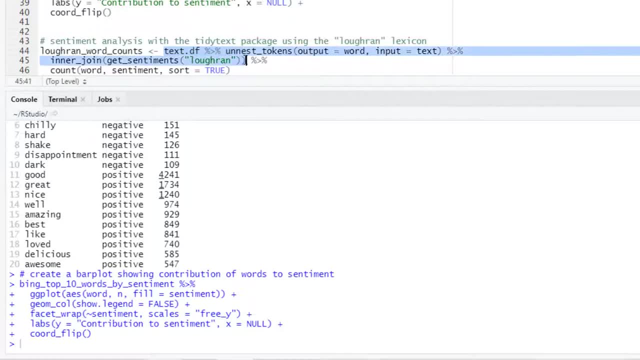 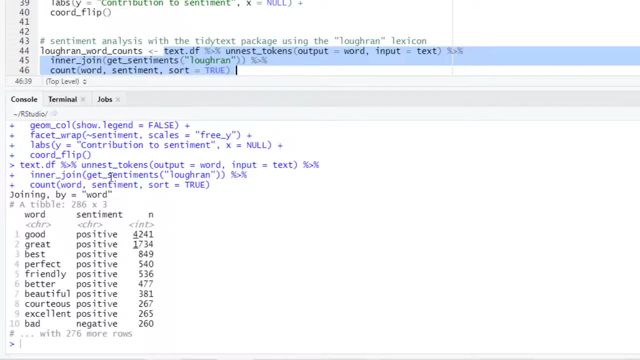 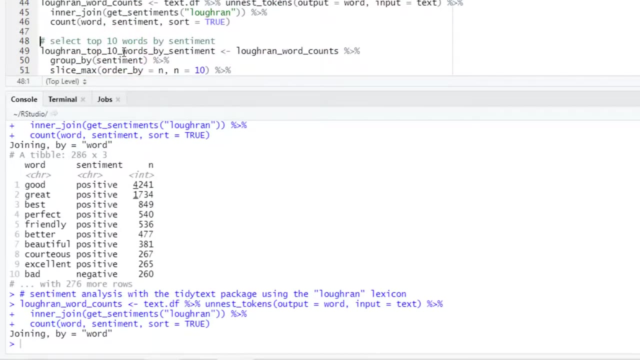 will do the join with the low brand lexicon and then we calculate the frequency for each of the words. So we can see now another table with three columns: the word in the first column, sentiment in the second column and the frequency in the third column. We can 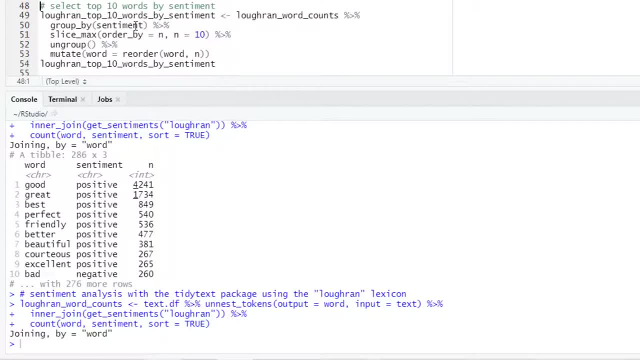 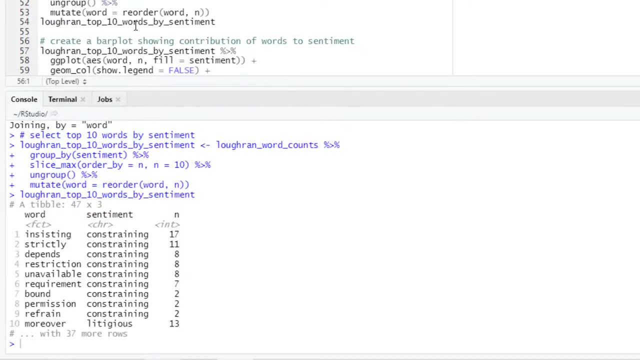 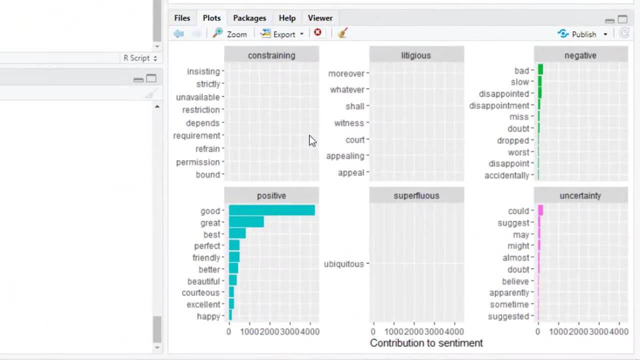 select the top 10 words by sentiment, as we did before, and we are going to get the top words for each of these sentiments and then we can create the visualization in a similar way. And here these are the sentiments in this lexicon, So we see constraining. 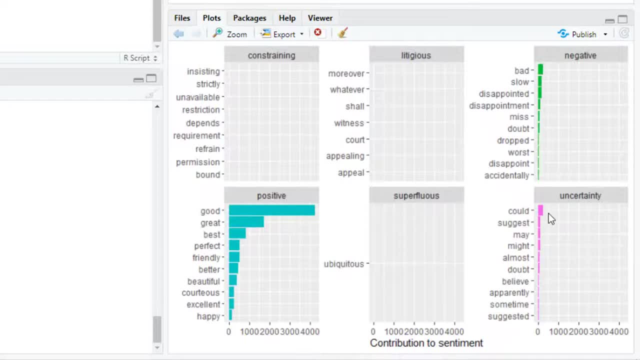 litigious, negative, positive, superfluous and uncertainty, And the words that we see in each of these facets corresponds to the words that are present in the text data set that were classified with the corresponding sentiment in this lexicon. Here most of the words for this data set about restaurant reviews.